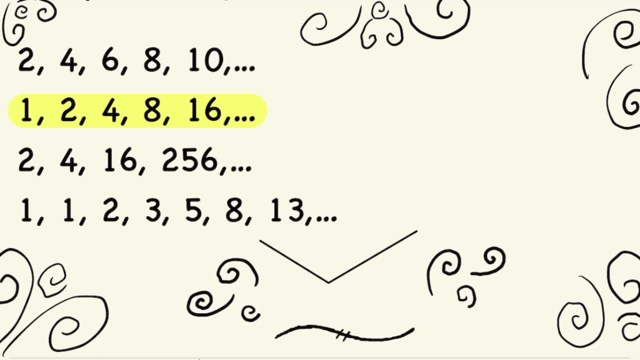 For this one, double the first number to find the second number. For example, eight times two is sixteen. The next number would be thirty-two. Next we have two, four, sixteen, two hundred and fifty-six. This one is a little harder. 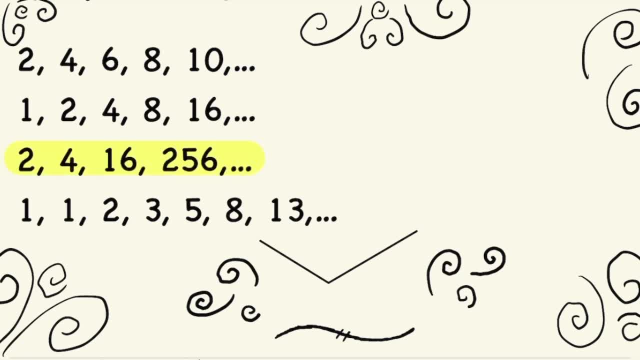 You have to multiply the first number by itself to get the next number. Sixteen times sixteen is two hundred and fifty-six. The next number would be sixty-five thousand five hundred and thirty-six, the square of two hundred and fifty-six. Finally, we have one one two. 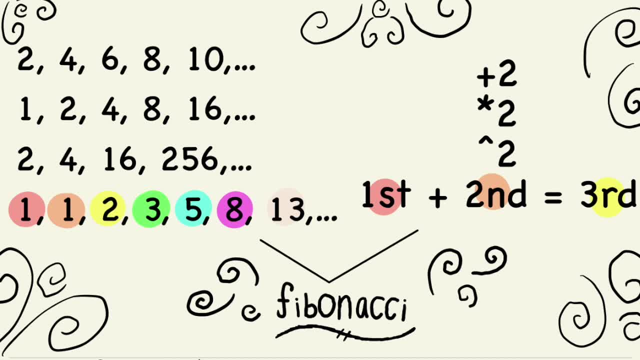 three and four. Next we have two, four, sixteen, two hundred and fifty-six. This one is a little harder. You have to multiply the first number by itself to get the next number. Sixteen times two is thirteen. The next number would be twenty-three, five, eight, thirteen. You can add two. 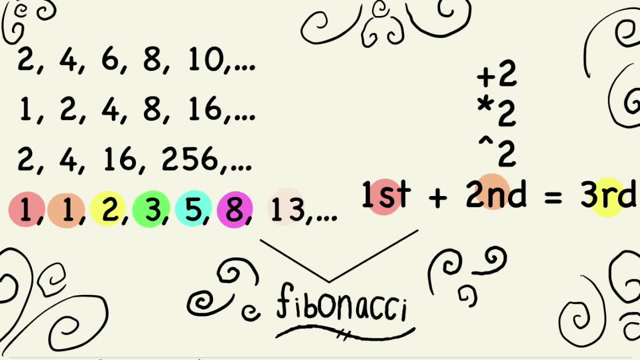 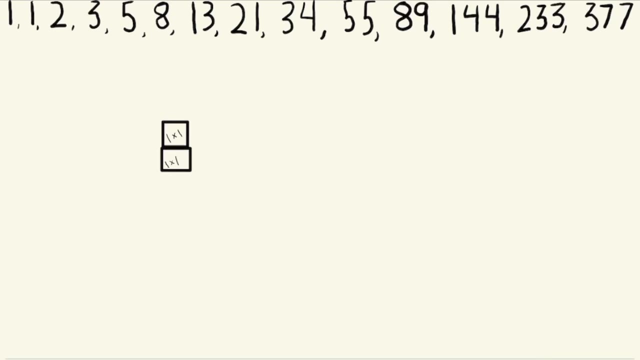 consecutive numbers to find the next. For example, five plus eight is thirteen, So the next number would be twenty-one, because eight plus thirteen is twenty-one. This pattern is the Fibonacci sequence. Now let's draw a spiral using these numbers. Start with two, one by one. 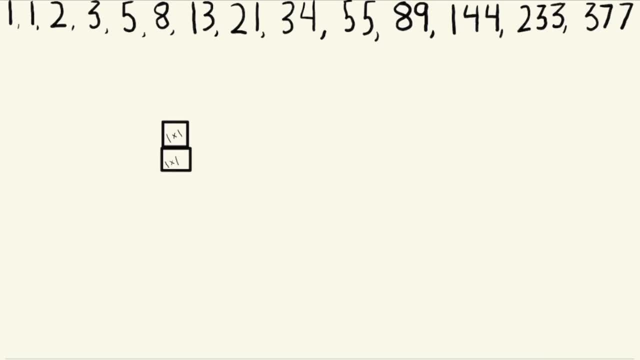 squares on top of each other, like so: Place a two by two square to the right of those Next, place a three by three above all of them, To the left of the one by ones. and three by three, draw five by five. Finally, place an eight by eight below all of them. It doesn't quite look. 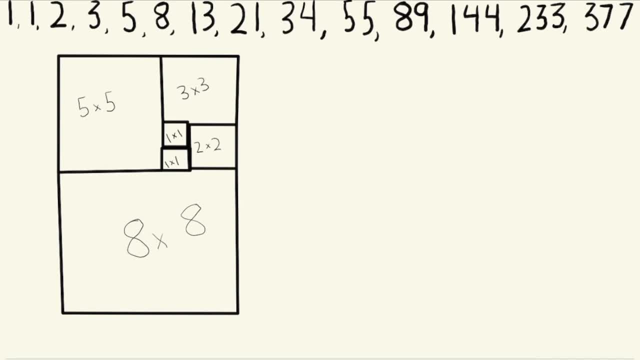 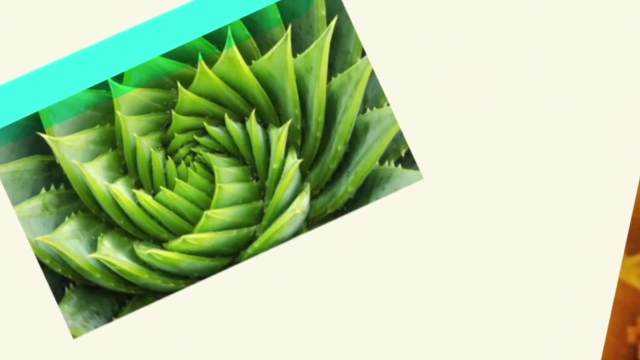 like a spiral yet. so add curves from corner to corner in each square. It should look something like this. So now we've learned how to draw a spiral, Now let's draw a spiral. So let's look at some examples in nature. First, this plant has one, two, three, four, five spirals. Hey, 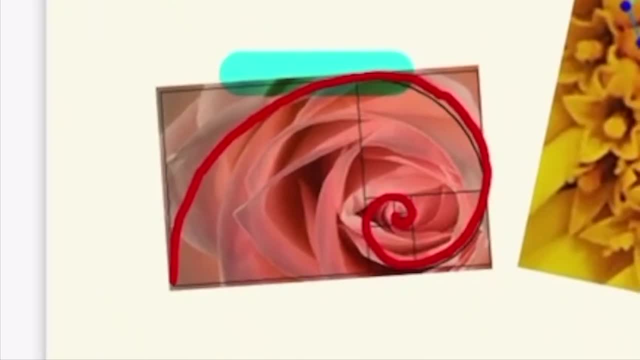 that's a Fibonacci number. This rose uses the Fibonacci spiral, created with a specific Fibonacci angle of one hundred and thirty-seven point five degrees in order to get the most sunlight in the smallest amount of space. So let's look at some examples in nature. First. this plant has one, two. 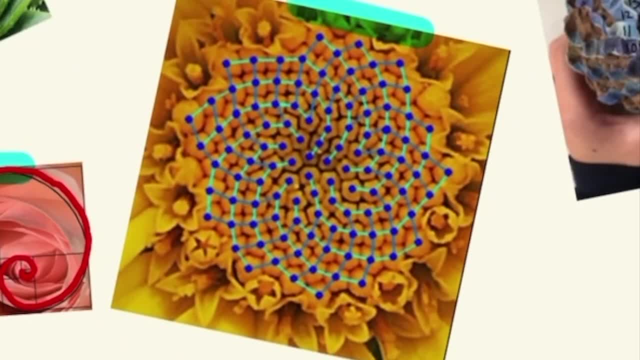 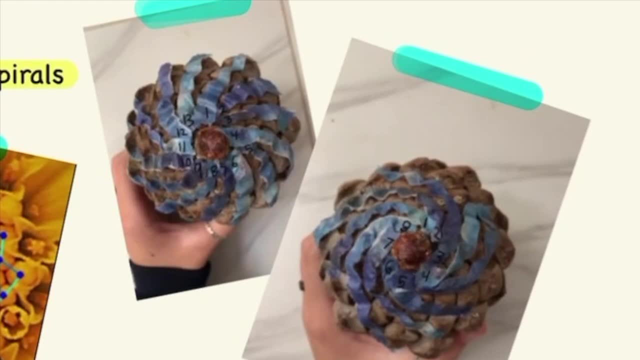 three, four, five spirals. This sunflower has thirteen spirals in one direction and twenty-one in the other. Those are Fibonacci numbers too. Or how about this pinecone that has thirteen spirals in one direction, just like the sunflower, and eight in the other? This sequence and spiral. 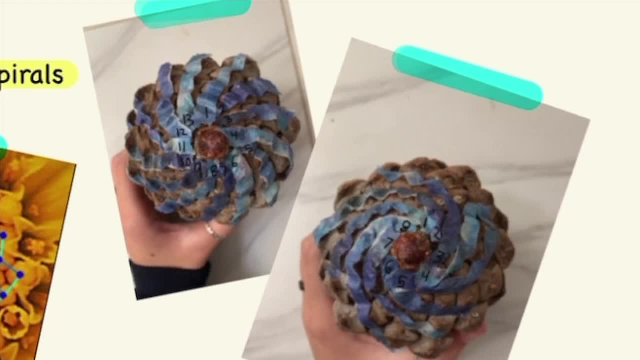 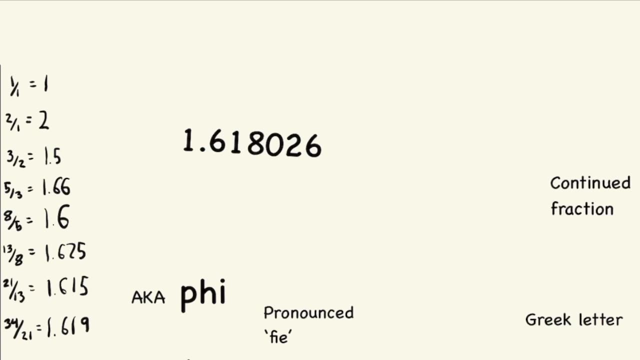 are found practically everywhere in nature. Can you think of any other places? But what's so special about this sequence? Let's look for a special ratio called the golden ratio. to find out, We can divide each number by the number before it to find a ratio. As we get further and 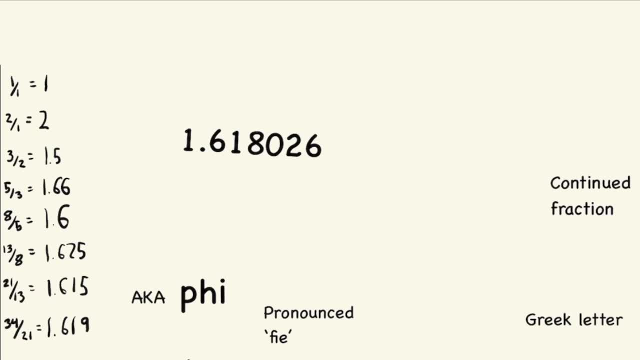 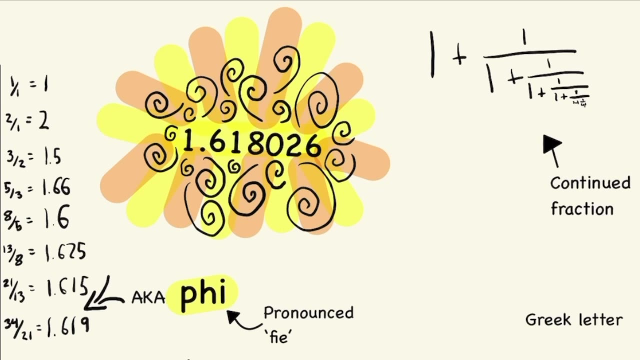 further in the sequence, the ratio gets more precise as it approaches a special number: One point six. one eight zero two six. We call this number phi. Phi is an awesome number because, unlike most numbers, phi cannot be approximated by a fraction, which means that even if you rotate, 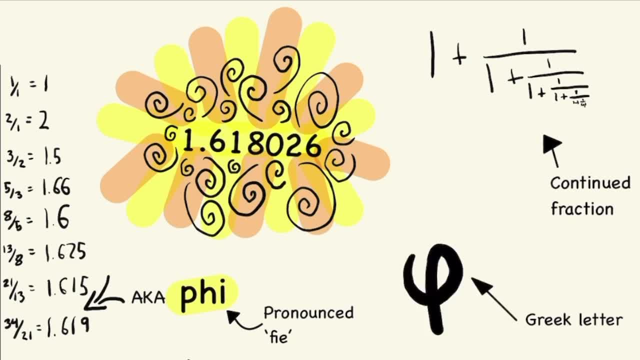 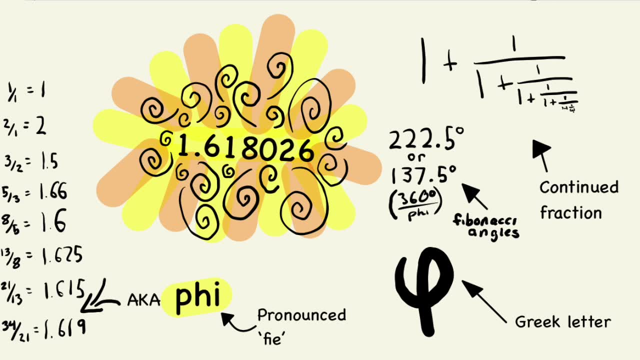 around a stem or center. you can't find a fraction. So we can't find a fraction because we can't find the ratio that fits our number, So we simply need to find an ratio. Uh, you can find some better variables for phi, like the number for the number, which means that it fits the answer. 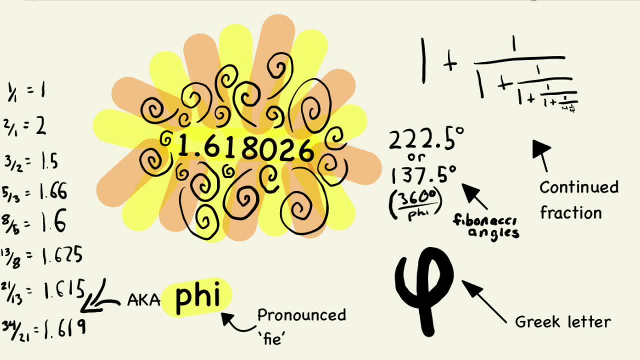 So this is the graph, This is what phi looks like, And it's comparatively common to find a ratio of one to twenty five times, and that's just the fact that you can't see how many different values that are related to the value of a number. So here we have two short values. 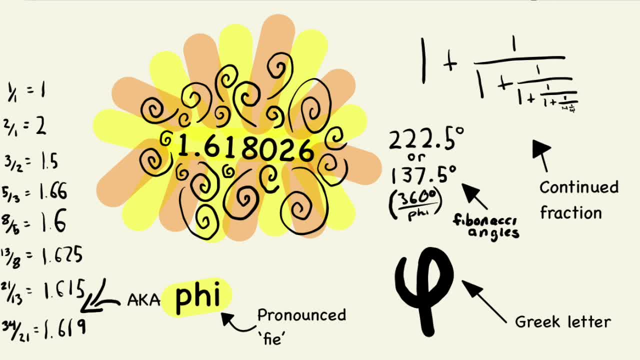 here, and then we have two, and we have one, and we have one, and we have two And we can see this as a number. so we'll only be able to see the ratio here. So let's find a ratio of one to twenty five times. We can see this as a number. So let's say: if I want this number, 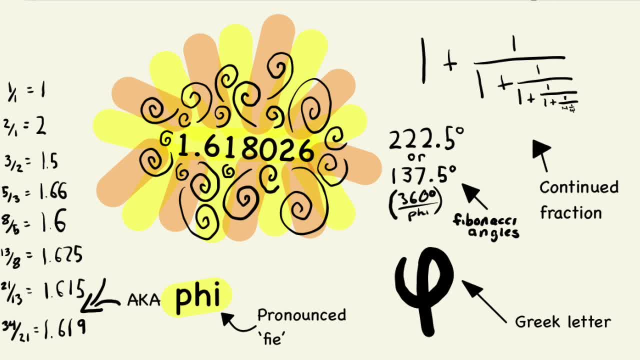 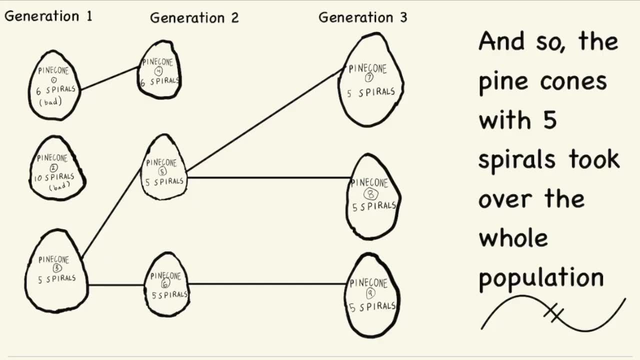 called the continued traction. here Also the two Fibonacci angles, which together sum to 360 degrees, can be seen here. So how do plants find phi? In short, evolution. Imagine you have three pine cones. The first one we'll make this. one orange has six spirals. It's fairly efficient. It reproduces once. 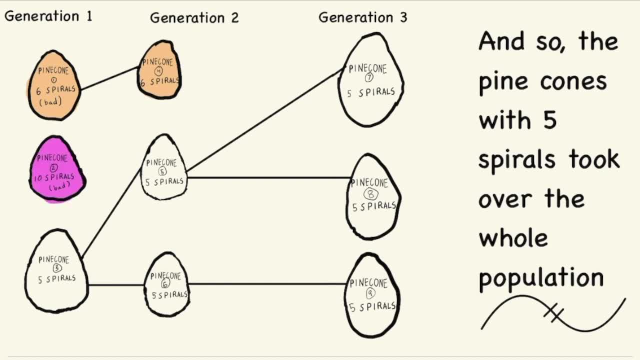 The second pine cone, the pink one, has 10 spirals, which is nowhere near a Fibonacci number. It doesn't reproduce at all, because it's nowhere near the golden ratio either. But imagine: your third pine cone has five spirals, a Fibonacci number and therefore a perfect.